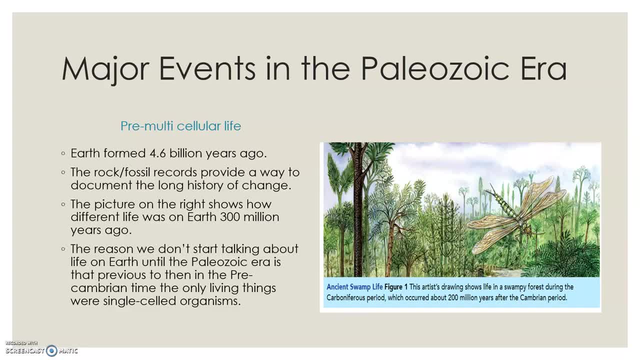 there, and I bet some of you know what that is: It's a dragonfly. It's a dragonfly. It's a dragonfly. Some of you can remember the dragonfly that I have in my classroom in the case and how big we. 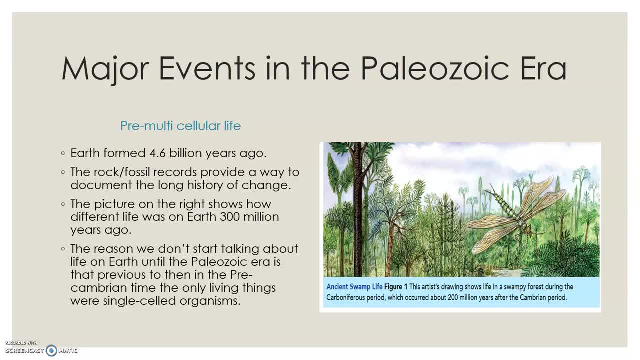 thought that one was, but we once drew on the board that some dragonfly's wingspans were even larger than our armspans, which is kind of crazy. So the reason we don't start talking about life on Earth until the Paleozoic era is previous to that, In the pre-Cambrian times, the only things 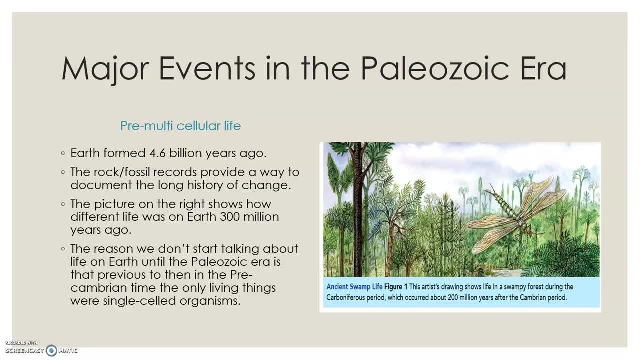 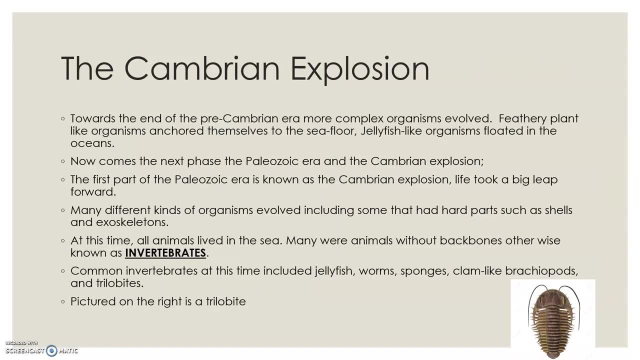 that were living were single-celled organisms, and the single-celled organisms were the single-celled start of the evolution of some multicellular organisms. So let's hop right into the Cambrian explosion. Towards the end of the pre-Cambrian era, more complex organisms evolved- Feathery. 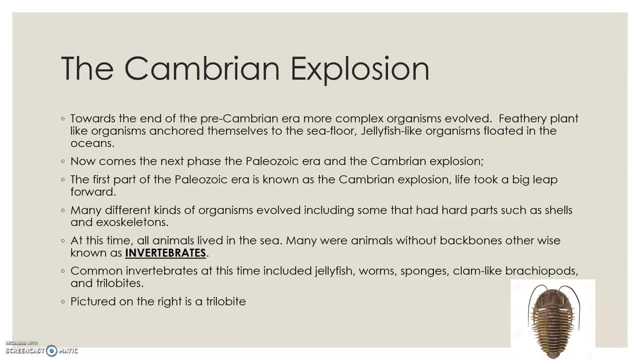 plants-like organisms anchored themselves to the seafloor, Jelly-like organisms which weren't exactly jellyfish floated in the ocean. Now comes the next phase, the Paleozoic era and the Cambrian explosion. The first part of the Paleozoic era is so crucial and important. 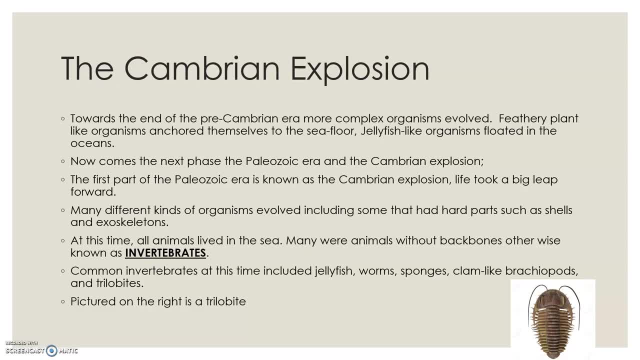 It's known as the Cambrian explosion, because life took a huge leap forward. during this time, Many different kinds of organisms evolved, including some that had hard parts, such as shells and exoskeletons, But at this time, all animals lived in the sea, Many animals without. 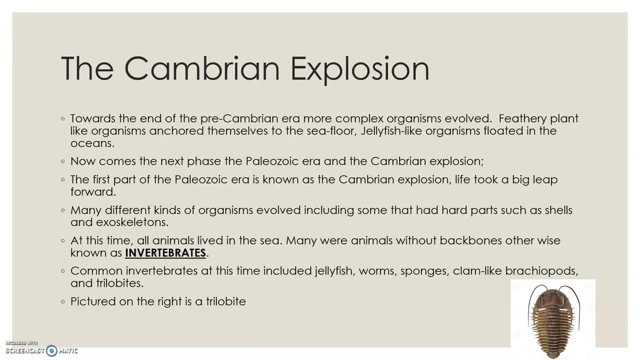 backbones, otherwise known as invertebrates, which you should know- excuse me, common invertebrates at this time included now the actual jellyfish, worms, sponges, clam-like brachiopods and tribolites. On the right there is a picture of a tribolite. 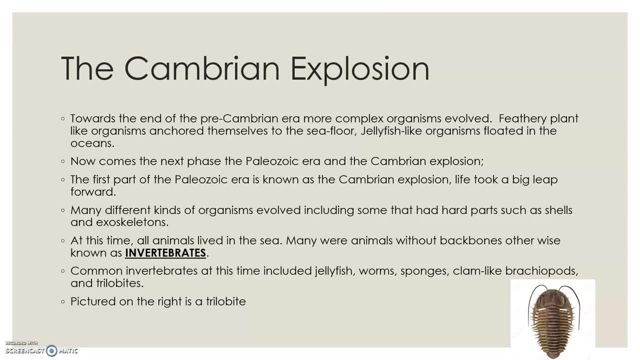 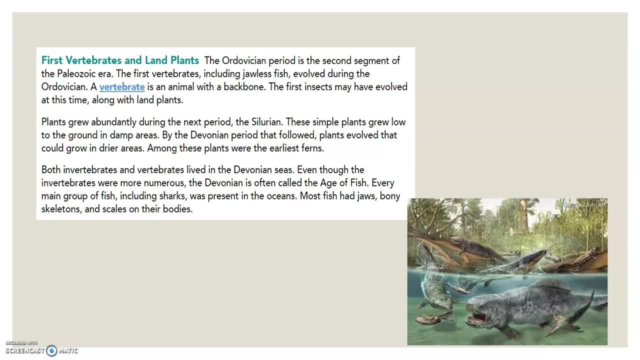 kind of like a horseshoe crab with antennae. Now the Ordovician period, the second segment of the Paleozoic era. Remember that eras are huge time spans broken down into smaller time segments, known as periods. Well, the Ordovician period. here is the second segment And here is 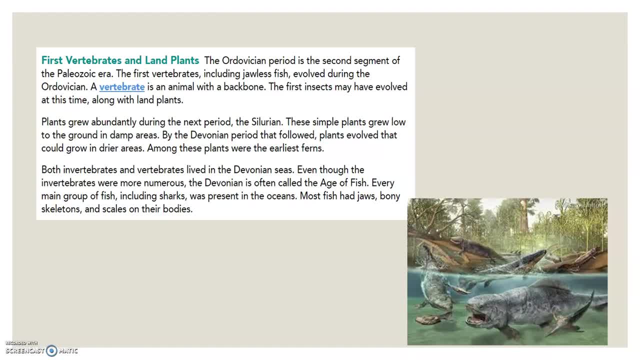 the first vertebrates, including jawless fish that evolved during this time, and vertebrates or animals with backbones. The first insects may have evolved at this time too, along with the land plants. Those land plants are going to become important very soon. Plants grew abundantly during 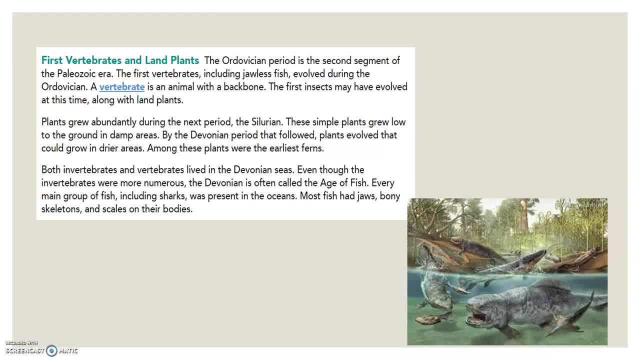 the next period, which was Silurian. These simple plants grew low in the sea, but they grew high in the sea. Plants grew low in the sea, but they grew high in the sea. Plants grew low in the sea, but they grew high in the sea. 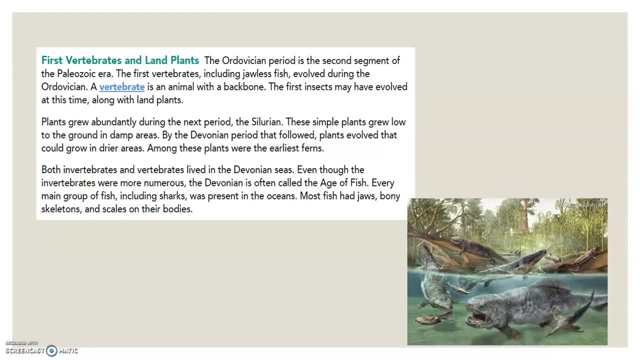 Plants grew low to the ground in damp areas. By the time we get to the Devonian period that followed, plants evolved that could grow in drier areas. So because of this, they were now diversifying so that they weren't just near swamps or bodies of water. So here were our first ferns. 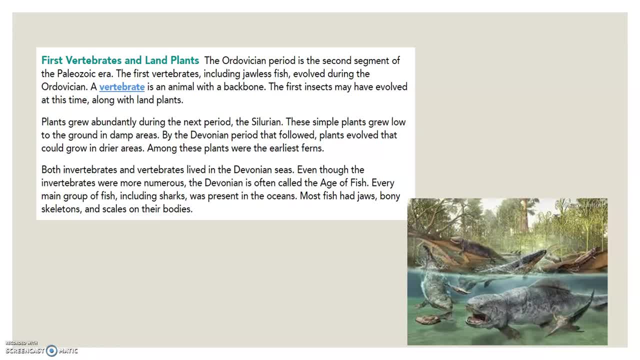 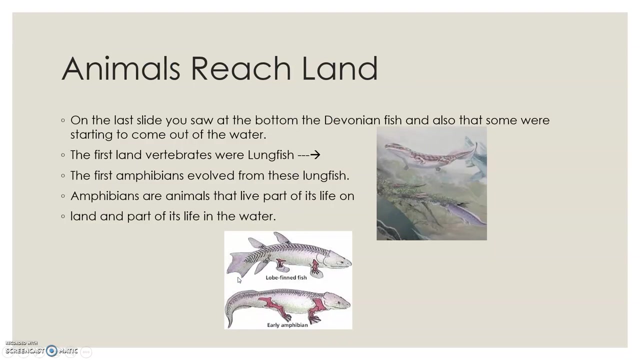 Now, both invertebrates and vertebrates did live during this time in the Devonian seas, Even though the invertebrates were more numerous. the Devonian period is a very long period of time, In fact. the Devonian period is often called the age of fish. Every main group of fish, including sharks, was present in the ocean. Most of these fish had jaws, bony skeletons and scales on their bodies. You can see, there on the right we have these creatures that have sort of legs. They look kind of like fish, kind of like crocodiles, and that's because their evolution was occurring. Now we've got the animals reaching land. 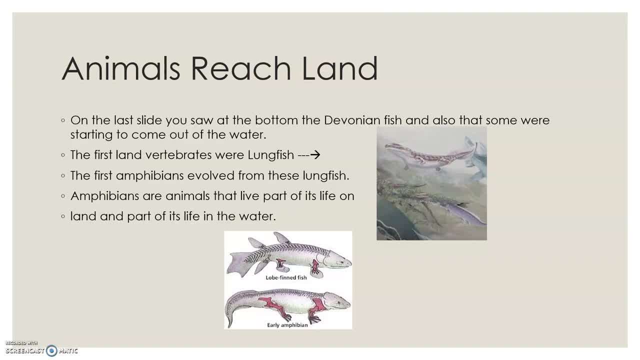 On the last slide you saw that the bottom of the Devonian fish and also some were starting to come out of the water. So the first land vertebrates were lungfish, pictured here on the right kind of a cross between, like a crocodile, alligator and a fish, The first amphibians. 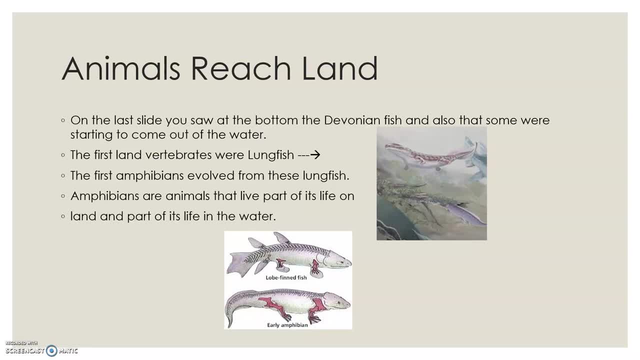 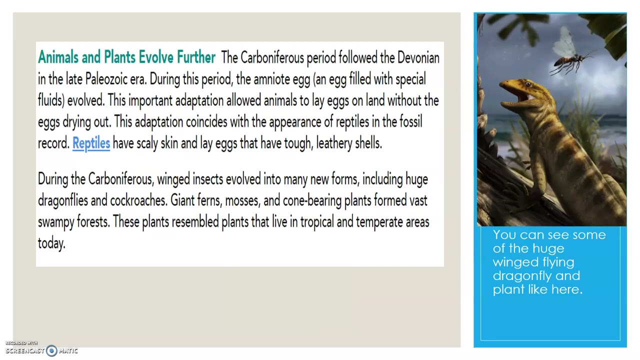 evolved from these lungfish and amphibians are animals that live part of their life on land and part of their life on water. So you can see the early amphibians directly came from these lobed, thin fish. You'll notice structural changes. Now we've got animals and plants evolving, even. 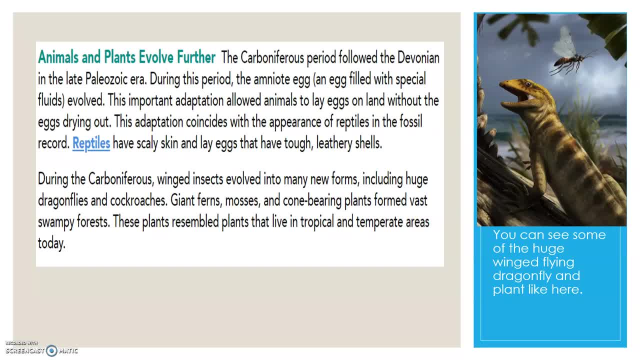 further. So now we go into the Carboniferous again, because we're all carbon-based life forms. This followed the Devonian period in the late Paleozoic era. during this period, the Amnesia period, neonite egg, which is an egg filled with special fluids. of all This adaptation was huge because 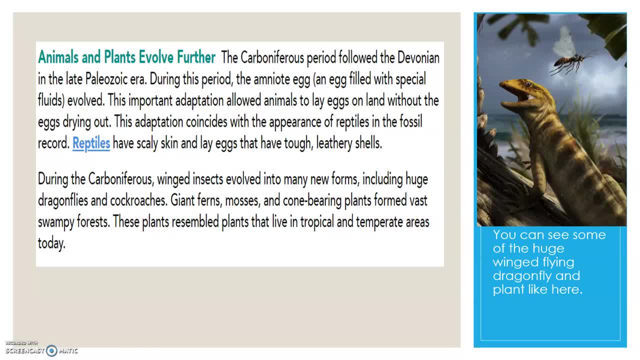 it allowed animals to lay eggs on land without the eggs drying out. This adaptation coincides with the appearance of reptiles, Again, reptiles being animals that have scaly skin and lay eggs that have tough leathery shells. During the Carboniferous period, winged insects evolved. 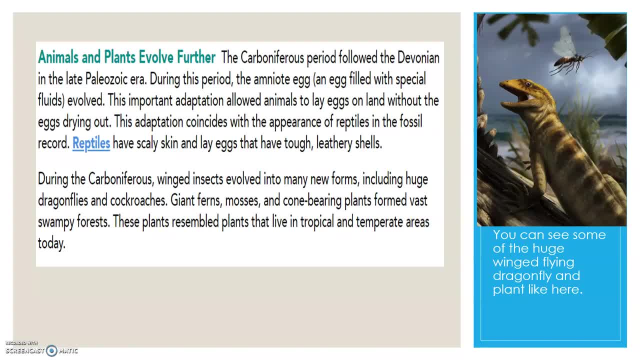 into many new forms, including huge- huge again, back to longer than our arm span- dragonflies and cockroaches the size of mice, Giant, ferns, mosses and cone-bearing plants formed vast swampy forests, And these plants resembled plants that lived in tropical and temperate areas today, 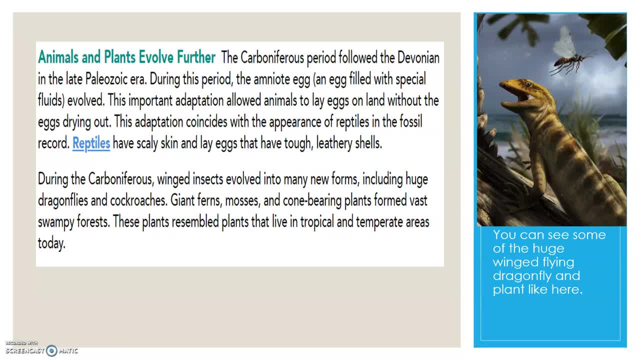 You can see some of the huge winged flying dragonflies and plants here, and this was probably one of them. This is one of the first reptiles that lived on land, But again, use his head as a reference for how big those flying bugs really were. Now we get to talk about Pangea right The Earth. 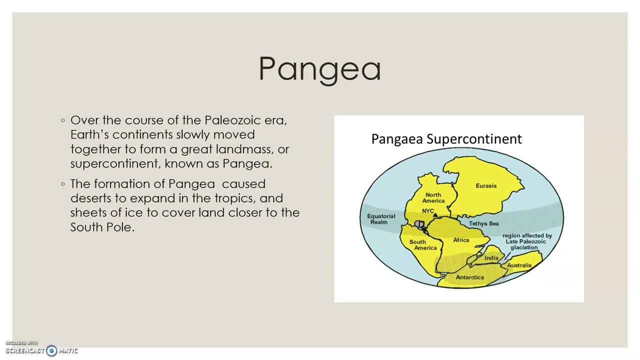 as one large mass right. It looks almost like a puzzle piece. Over the course of the Paleozoic era, Earth's continents slowly moved together to form a great landmass or supercontinent. The formation of Pangea caused deserts to expand in the tropics and sheets of ice to cover land. 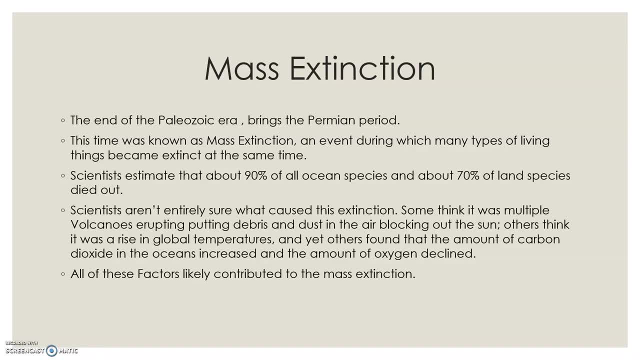 closer to the South Pole. Then we talk about mass extinction. The end of the Paleozoic era brings the Permian period. This time was known as mass extinction, an event during which many types of living things became extinct at the same time. Scientists estimate that about 90% of all 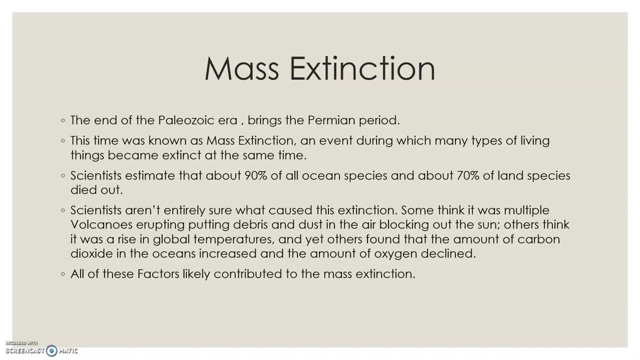 ocean species and about 90% of all living things became extinct. at the same time, About 70% of land species died out. Scientists aren't exactly sure what caused this mass extinction. It could have been multiple volcanoes erupting putting so much debris and dust into the air. 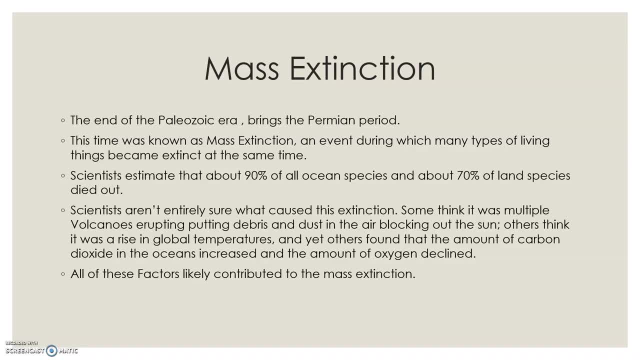 blocking out the sun. Well, when you block out the sun, that obviously is going to change the temperature and not allowing plants to grow. Others think it was a rise in global temperature, and yet others found that the amount of carbon dioxide in the oceans 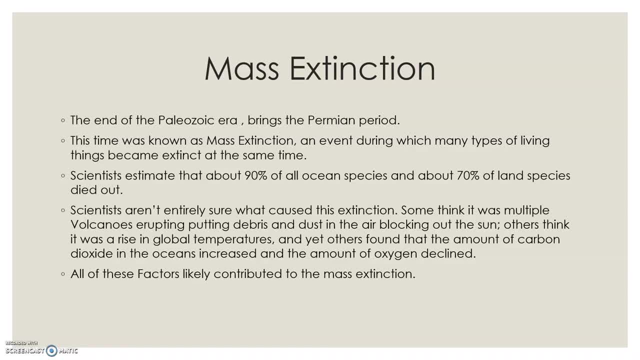 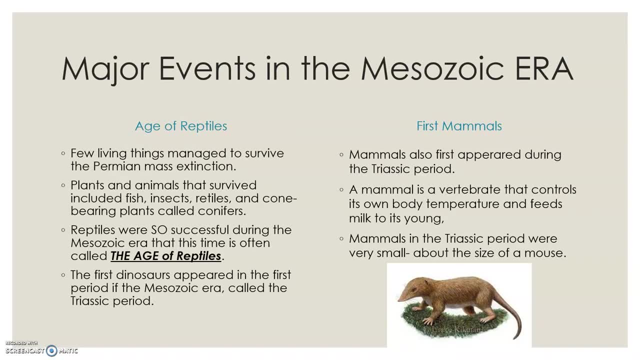 and therefore the amount of oxygen declined. But very likely all of these factors likely contributed to the mass extinction. Now we move into the next major time era. Again, the larger blocks And these are the major events in the Mesozoic era. We've got our age of reptiles. 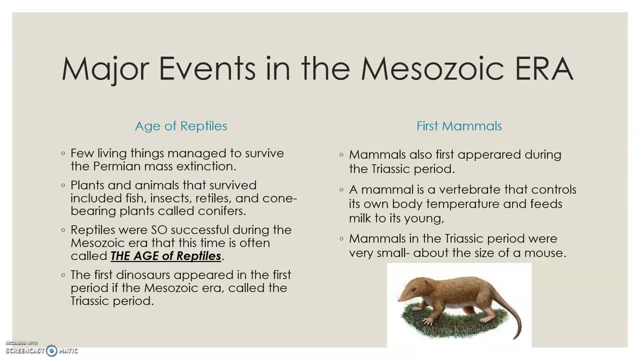 We go back to the mass extinction Few living things managed to survive the Permian mass extinction, but the plants and animals that did survive included the fish, insects, reptiles and cone-bearing plants called conifers. The reptiles were so successful during the Mesozoic era that 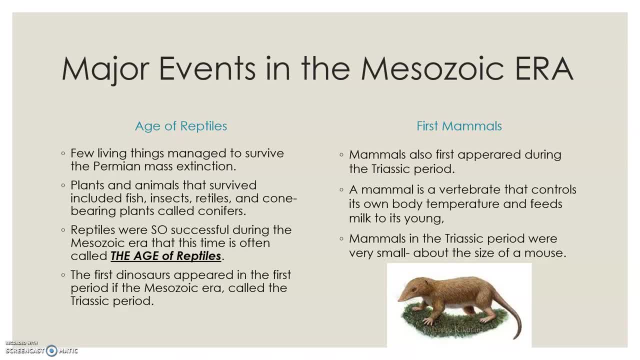 this time is often called the age of reptiles. The first dinosaurs appeared in the first period in this Mesozoic era called the Triassic period, And then we also have our first mammals occurring during the Triassic period. And then we also have our first mammals occurring during the Triassic period. 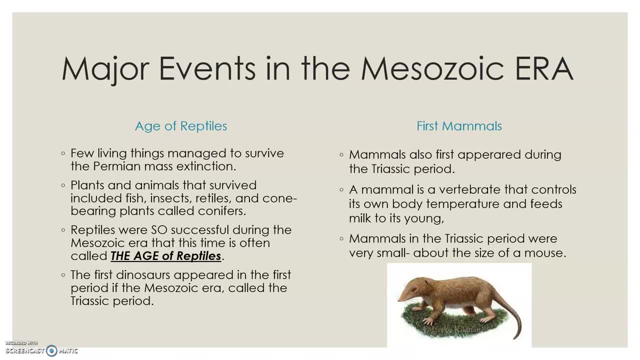 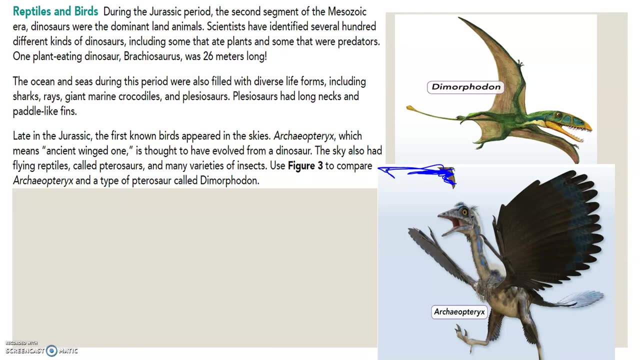 A mammal is a vertebrate that can control its own body temperature and feed milk to its young. Mammals in the Triassic period were very small, only about the size of a mouse like this cute little fella here. Then we get to these scary reptiles and birds. 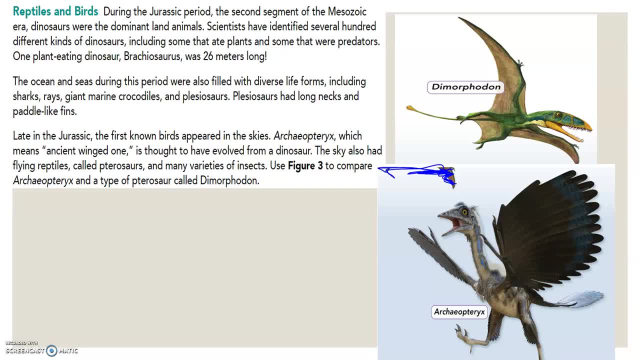 During the Jurassic period, which is probably the period you guys have heard the most about, which is the second segment of the Mesozoic era, dinosaurs were the dominant land animals, And scientists have identified several hundred different kinds of dinosaurs, including some that ate plants and some that were predators. 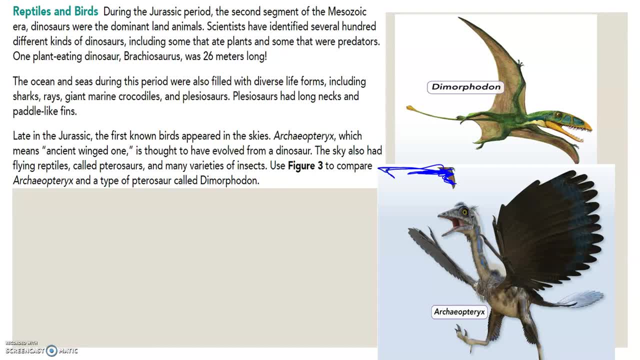 One plant-eating dinosaur, Brachiosaurus, was 26 meters long. The ocean and the seas during this period were also filled with diverse life forms, including sharks, rays, giant marine crocodiles and plesiosaurs. Plesiosaurs had long necks and paddle-like fins. 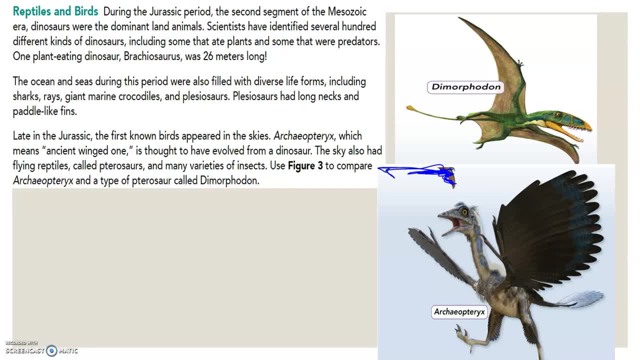 Late in the Jurassic, the first known birds appeared in the sky. This type of Archaeopterix- sorry, which literally means ancient winged one- is thought to have evolved from a dinosaur. The sky also had flying reptiles called pterosaurs and many varieties of insects. 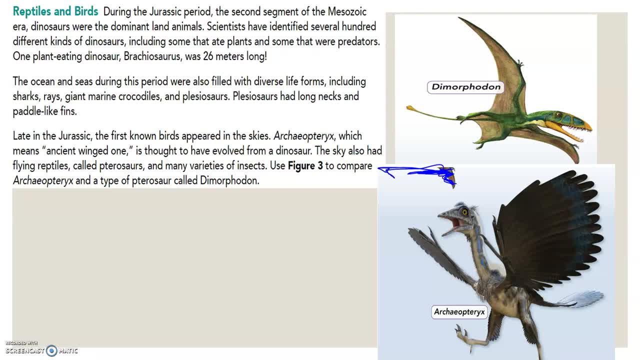 So if you look at these two here, we can see how the Archaeopterix and the Dimer the Archaeopteron- sorry I'm terrible with dinosaur names, but you can see how one could be able to be suited for more for land and one more for the air. 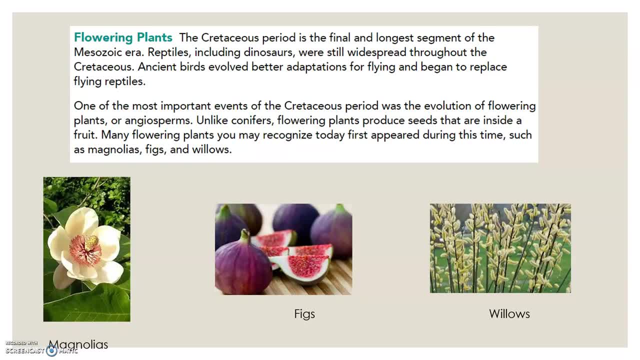 Then we get to our flowering plants. This is in the Cretaceous period. It's the final and longest segment of the Mesozoic era. The reptiles, including dinosaurs, were still widespread. Ancient birds evolved better adaptations for flying And- one of the most important things that happened to the Archaeopteris. 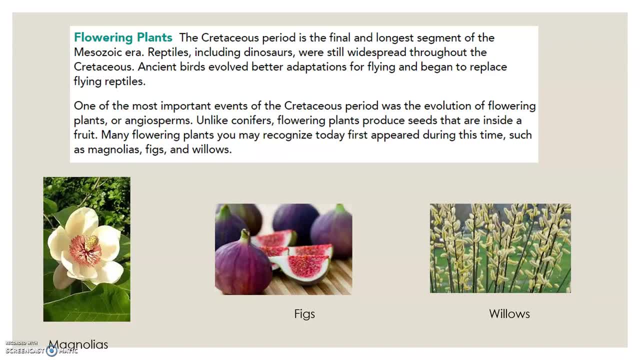 which is the one that happened here, was the evolution of flowering plants, otherwise known as an angiosperm. Unlike conifers, the flowering plants now are producing seeds that are inside of fruit, So this gave more variety of foods to the species existed. 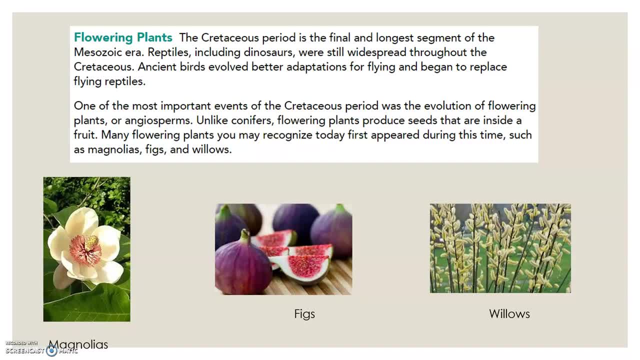 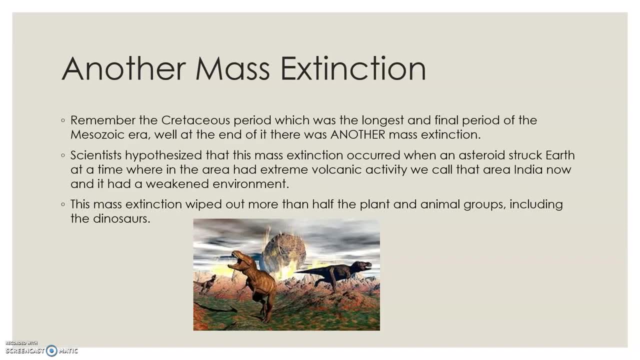 Some of the things that came out of it that we still recognize today are magnolias, figs and willows. We have another mass extinction: Run dinosaurs, run, Run dinosaurs run. A huge asteroid may have come down and this caused a lot of volcanic activity. 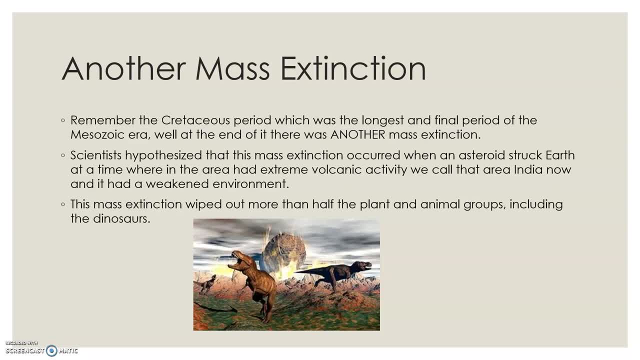 in where we would call India now, and it had a weakened environment. This again wiped out more than half plants and animal groups, including the dinosaurs- Bye-bye dinosaurs. So then, lastly, we move into the Cenozoic era. 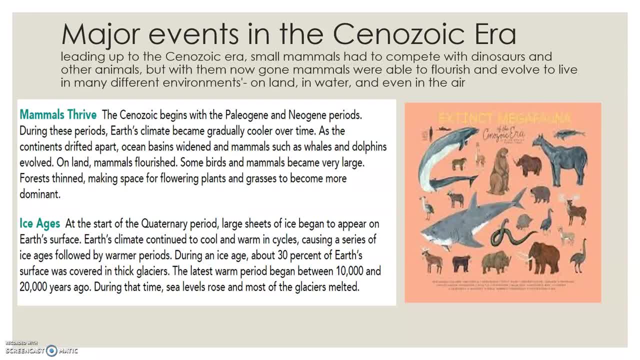 Now leading up to the Cenozoic era, we talked about those small mammals, but they had to compete with dinosaurs and other animals. But with them now gone, mammals were able to flourish and evolve to live in many different environments on land. 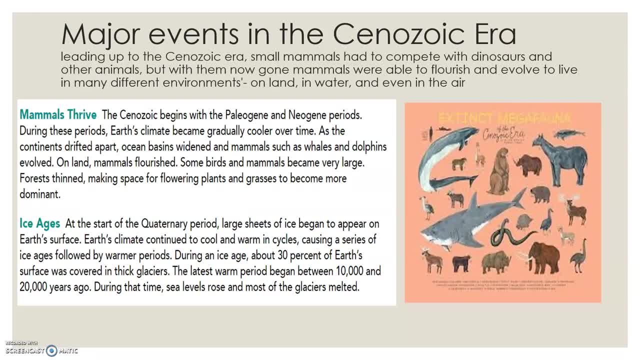 in water and even in the air. So this is the Cenozoic era begins with Paleogene and Neogene period. The climate cooled over time, We had whales and dolphins And then we've got the Ice Age at the start of the Quaternary period. 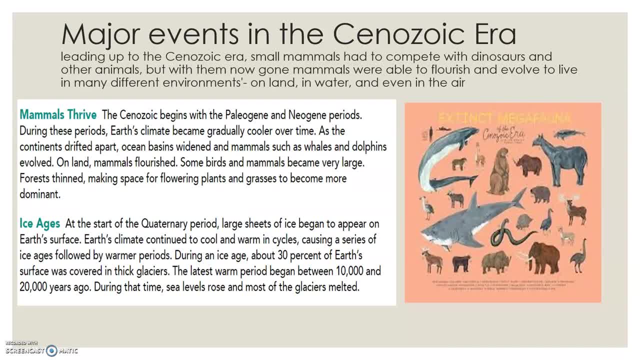 And then we've got the Ice Age at the start of the Quaternary period. And then we've got the Ice Age at the start of the Quaternary period. Large sheets of ice begin to appear on Earth's surface. Earth's climate continued to cool and warm in cycles.